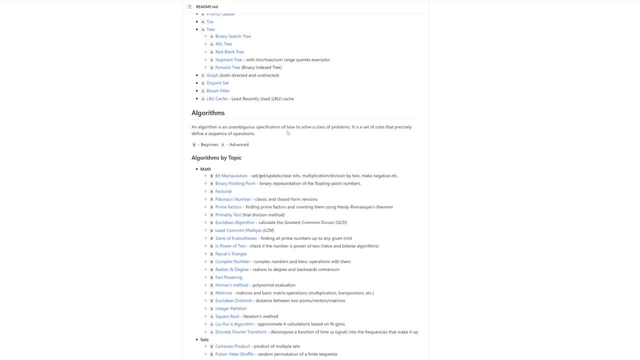 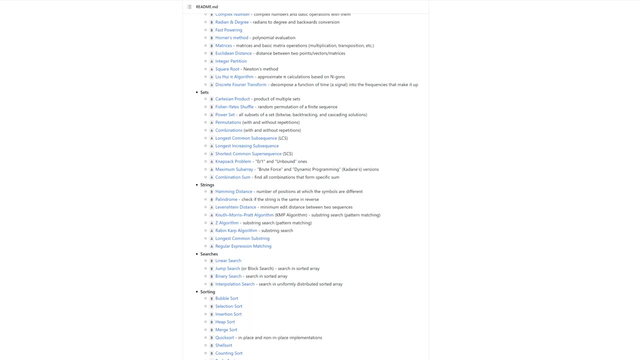 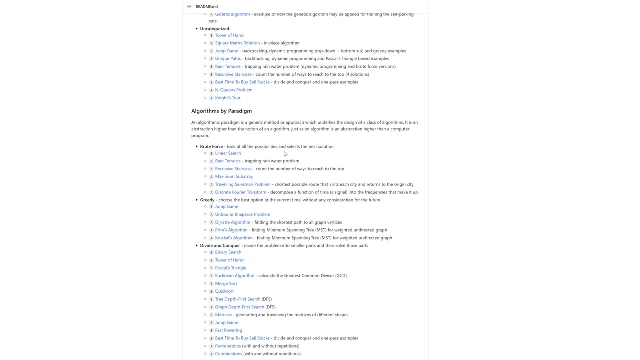 javascript developer is that there is not a lot of videos about this and algorithms, like you would see with Python, for example. so a repository like this is great because it has basically everything that you need and things that you wouldn't even find on YouTube. so, with that being said, I want to show you 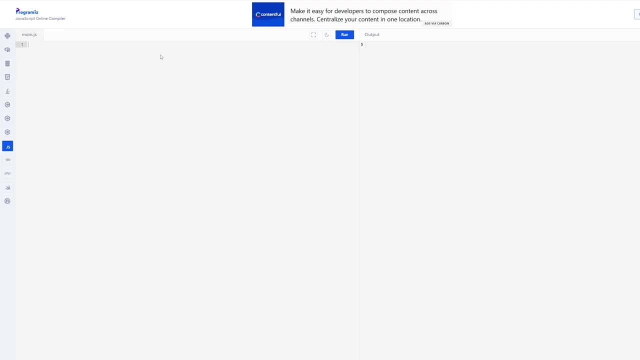 the implementation of the linear search and it's it's very simple, very easy to remember and very easy to implement into code as well. so we're gonna have our function and we're gonna call it linear search and we're gonna take an array and a key and basically the way that this algorithm works is just like I'm 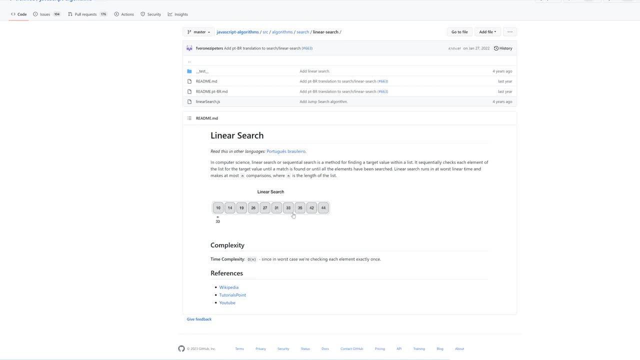 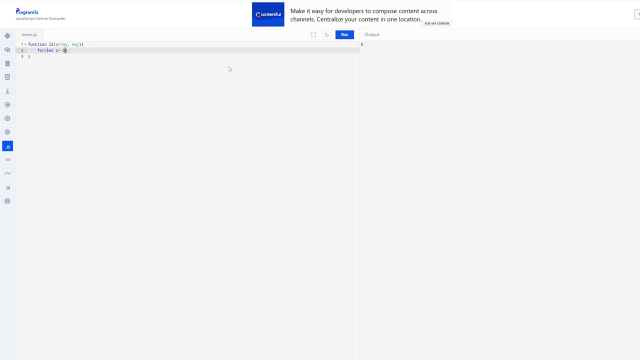 mentioned, it traverses through the elements of the array until it finds what it looks for and it has an average time complexity of O, which is pretty interesting. so we want to set, we basically want to traverse the array and we do it with a for loop and then we use an if statement and we say if the 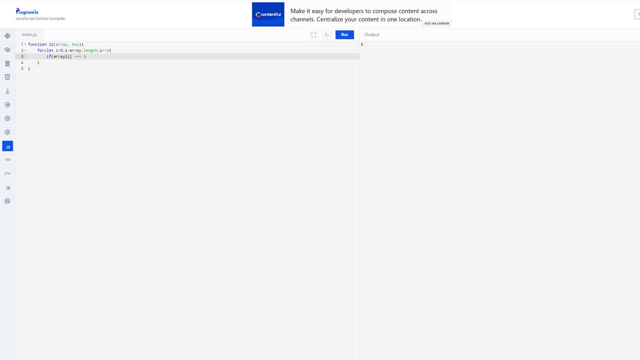 array at the i index is equal to the key, we want to return that element, and if it's not, we want to return minus one. pretty simple. now let's try it out. we're going to log it to the console and have a simple array with three elements. one, two, three, four, five, six, seven, eight, nine. and we're going to set it to the and have a simple array with three elements: one, two, three, four, five, six, seven. and we're going to set it to the console and have a simple array with three elements. 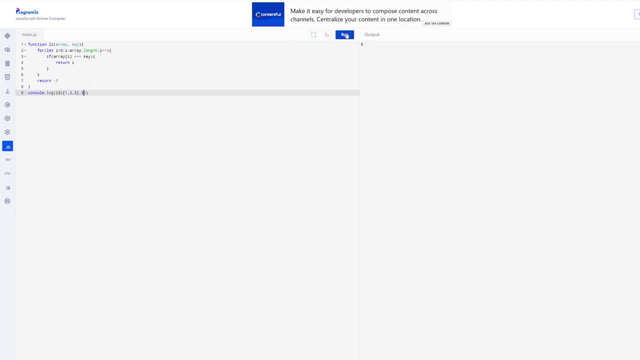 one, two, three and look for the third element or the the three in the array one, two, three and look for the third element or the the three in the array one, two, three and look for the third element or the the three in the array and, as we can see in here, it gives us two. 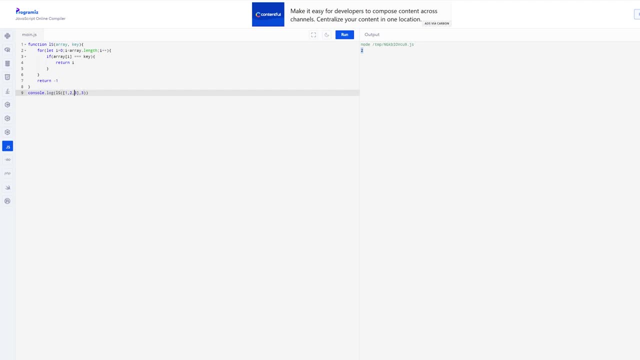 and, as we can see in here, it gives us two. and, as we can see in here, it gives us two because index zero one and two. the third, because index zero one and two. the third, because index zero one and two. the third element, like the element three, is in the. 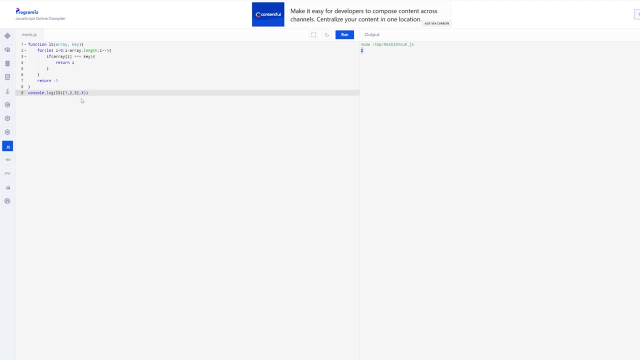 element, like the element three is in the element. like the element three is in the second element. like the second element. second element, like the second element. second element, like the second element of the array. now, what if we look for of the array? now, what if we look for? 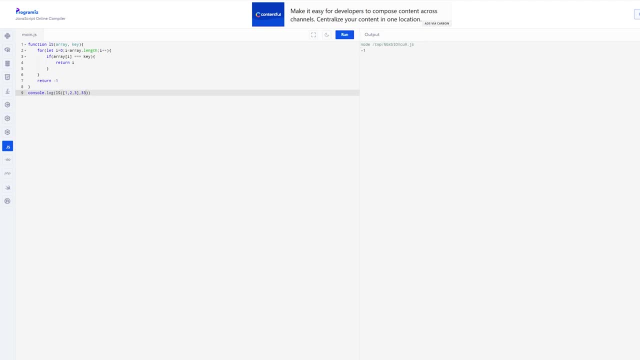 of the array. now, what if we look for something that's not in the array, for something that's not in the array, for something that's not in the array, for example, 33, example, 33, example 33. well, we're gonna get minus one, so it's yeah. that's basically the whole. 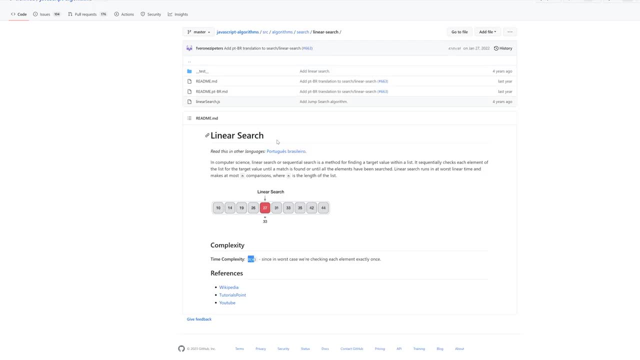 so it's: yeah, that's basically the whole. so it's: yeah, that's basically the whole point of point of point of: uh, this algorithm, uh this algorithm, uh this algorithm, and yeah, i hope you guys learned and yeah, i hope you guys learned and yeah, i hope you guys learned something today. i hope that you like. 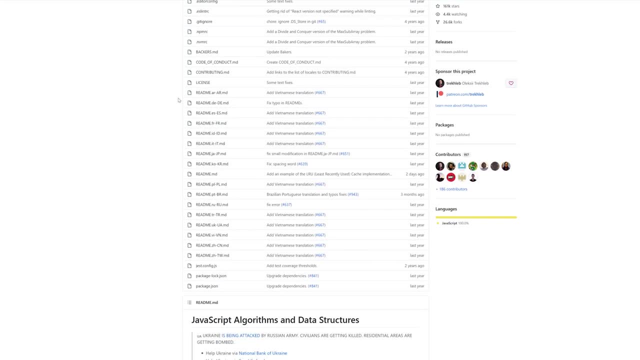 something today. i hope that you like something today. i hope that you like this video and the most important part. this video and the most important part. this video and the most important part is: don't don't stop learning. don't stop is don't don't stop learning, don't stop. 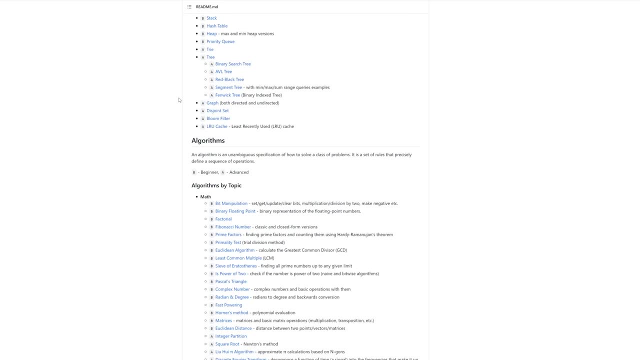 is: don't don't stop learning, don't stop studying, because if you want to become a studying, because if you want to become a studying, because if you want to become a software engineer, software engineer, software engineer, knowing the data structures and knowing the data structures and knowing the data structures and algorithms is very important. it comes up. 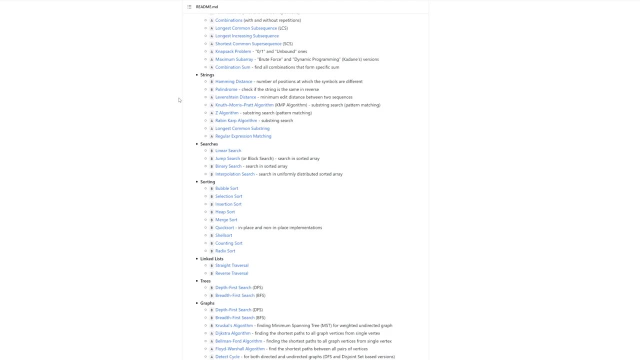 algorithms is very important. it comes up. algorithms is very important. it comes up in almost every full stack interview, in almost every full stack interview, in almost every full stack interview. so so so, that being said, hope you guys like it. that being said, hope you guys like it. 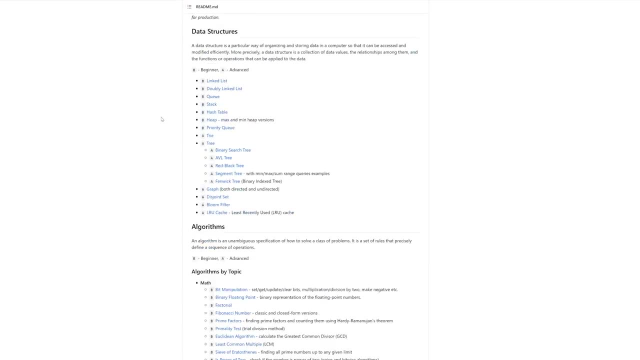 that being said, hope you guys like it. please take a look at the repository. and please take a look at the repository. and please take a look at the repository and learn everything that you need. if you learn everything that you need, if you learn everything that you need, if you like it, please thumbs up. 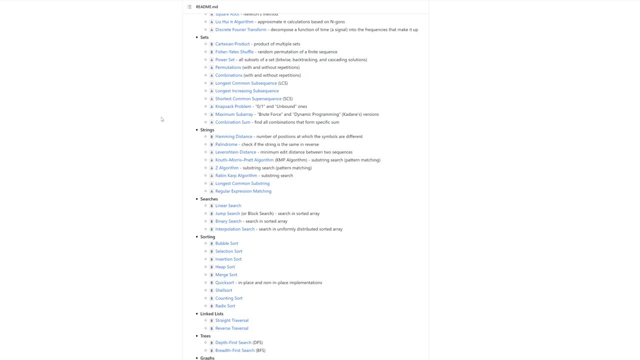 like it, please thumbs up. like it, please thumbs up and subscribe to the channel. and until the next one and subscribe to the channel. and until the next one, and subscribe to the channel. and until the next one. guys, peace out, guys, peace out.